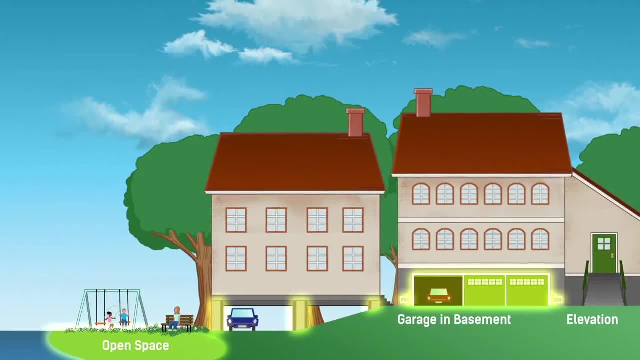 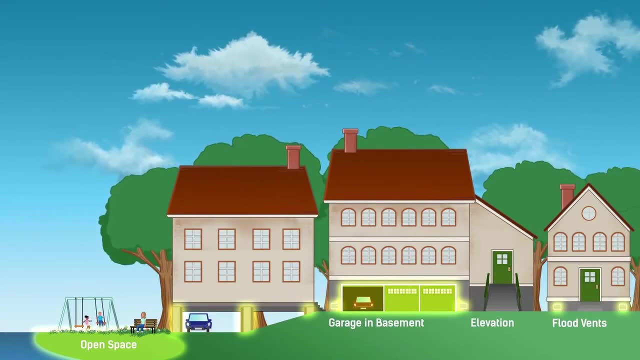 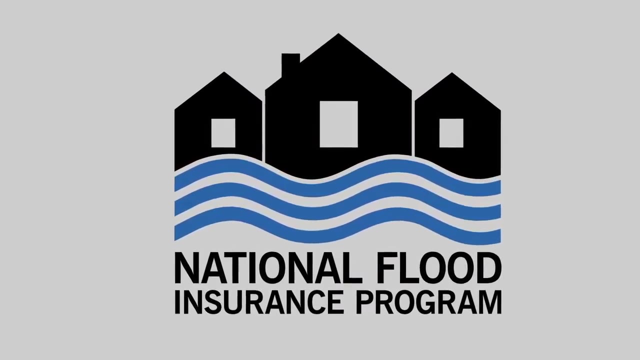 and promoting flood insurance. Many communities adopt and enforce even higher standards, which reduces damage from future floods and allows for quicker recovery. Communities that join the National Flood Insurance Program, or NFIP, agree to adopt and enforce floodplain management regulations. In return, they have access to federally-backed flood insurance. 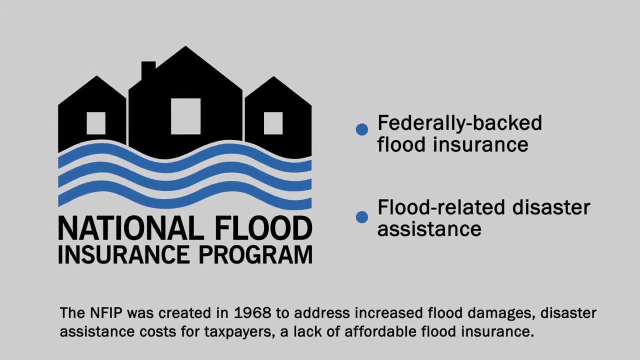 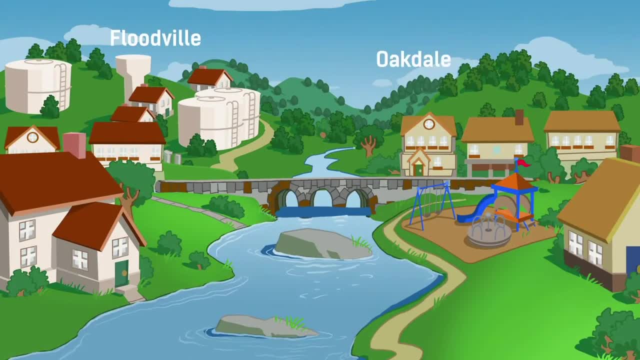 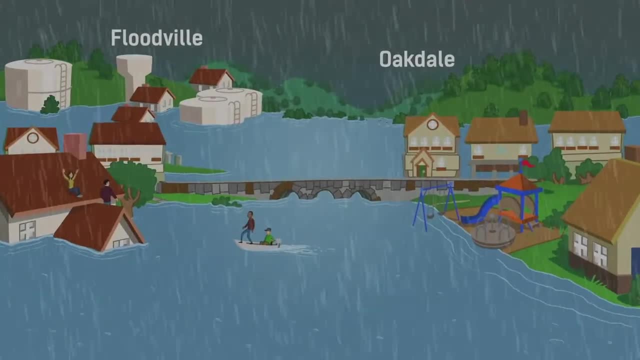 and flood-related disaster assistance and grants. So what happens to a community that doesn't practice floodplain management? Let's take a look. Floodville and Oakdale are neighboring towns. They each experienced heavy rainfall resulting in extensive flooding. Floodville did not join the 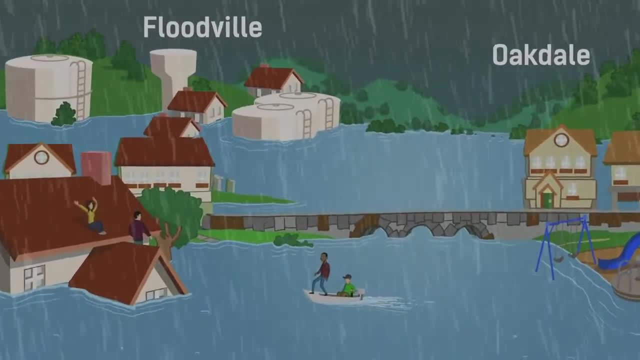 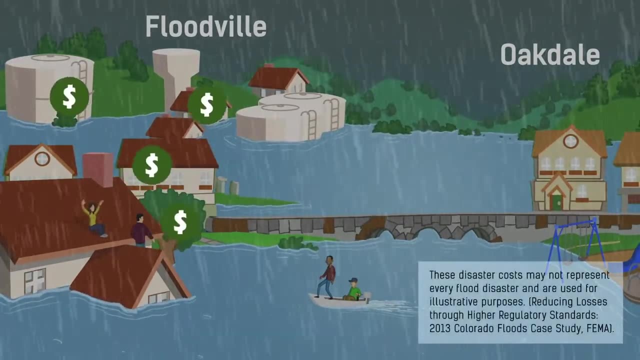 NFIP and did not adopt the required minimum standards to reduce their community's flood risk. Due to the lack of floodplain management requirements, Floodville's recovery costs were 40% more than Oakdale's costs, not to mention the financial impact on Floodville. 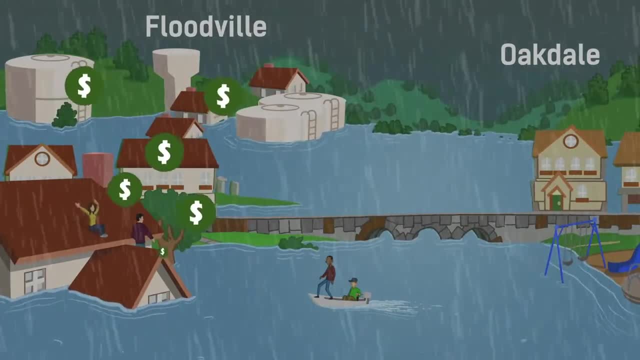 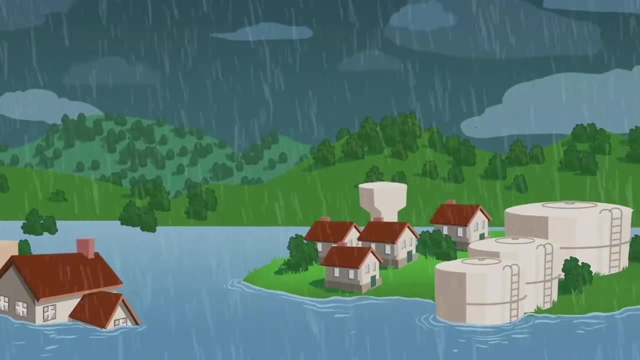 and its businesses, as it took so much longer to recover. Floodville's water treatment plant was damaged, while Oakdale's plant, built on high-pressure, was damaged. Floodville's water treatment plant, built on higher ground, was up and running the day after floodwaters receded. 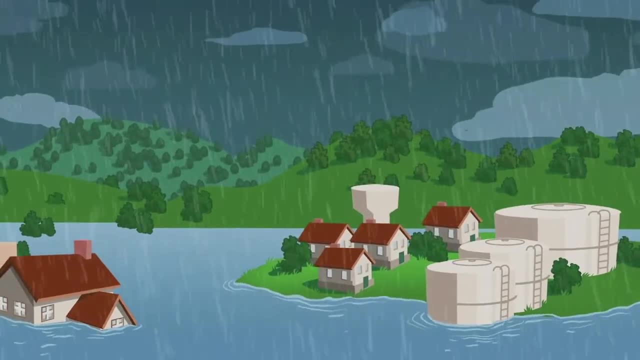 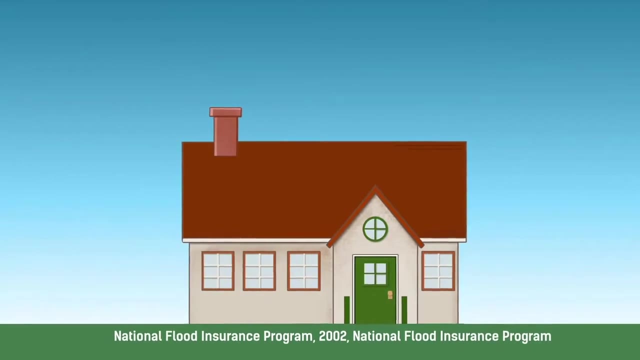 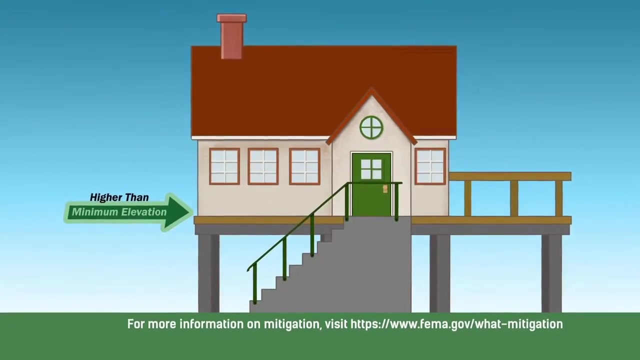 In addition, it was more difficult for Floodville's emergency services to respond, which put more lives at risk. Over the past 50 years, the NFIP has learned that buildings constructed after communities enforcing floodplain management regulations sustained about 80% less damage than those built before. 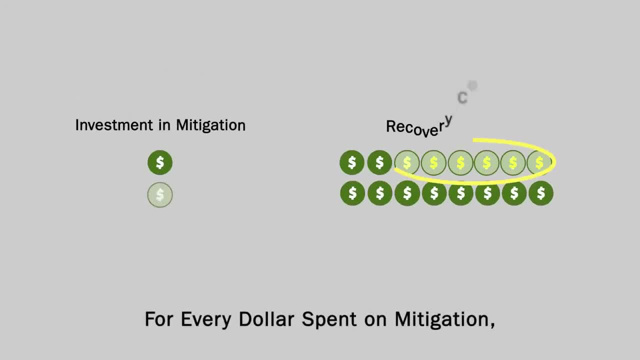 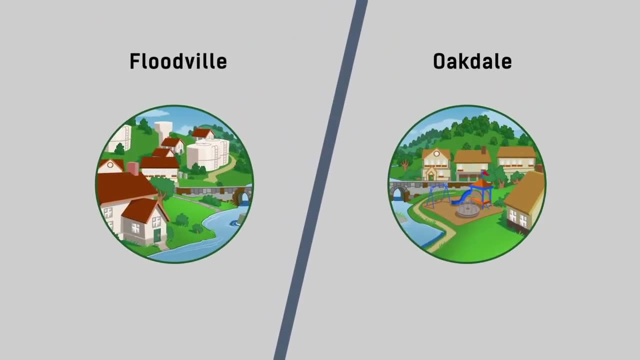 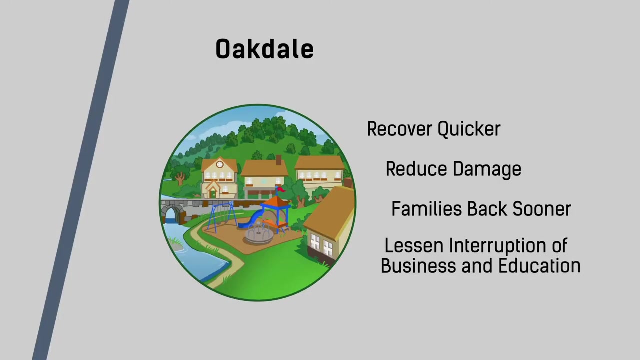 Research shows that for every dollar spent on mitigation, about six dollars are saved in future avoided losses. In short, communities like Oakdale are more resilient and recover more quickly. They save money, reduce further damage, get families back in their homes sooner and lessen business and 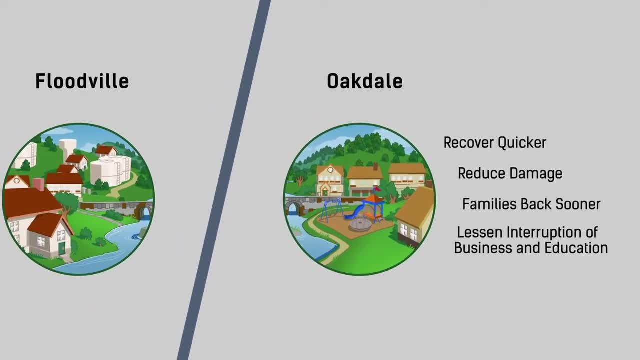 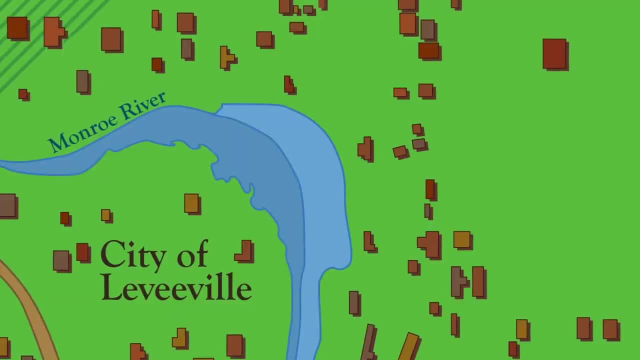 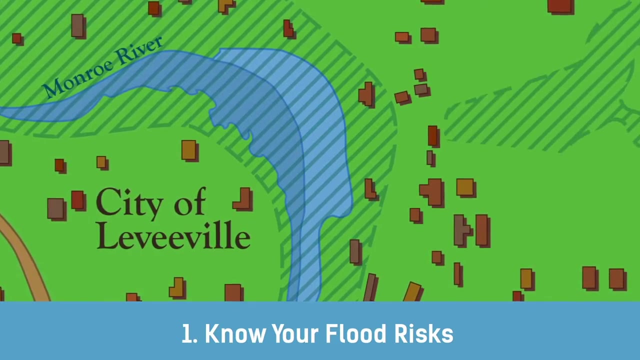 education interruption in their communities by practicing sound floodplain management. Here are a few simple steps to get started on floodplain management in your community. Know your flood risks. Are there homes or businesses that get flooded over and over Levees built before there were Chevys? 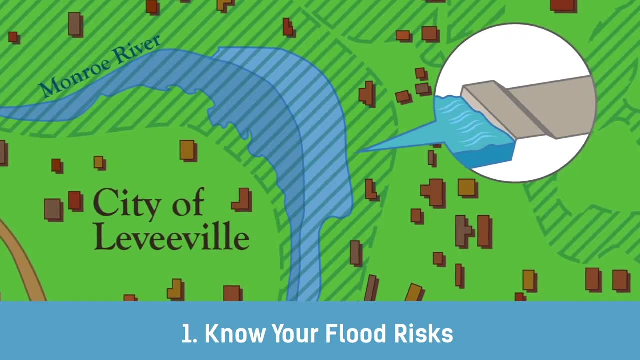 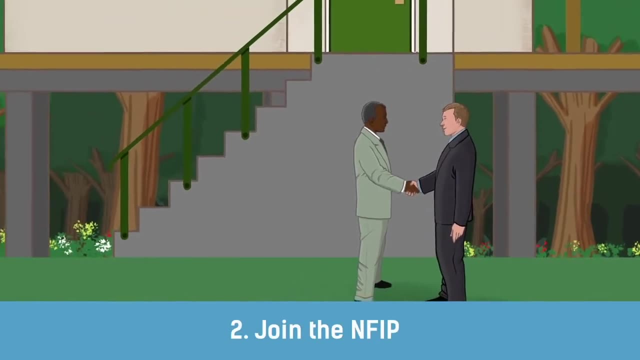 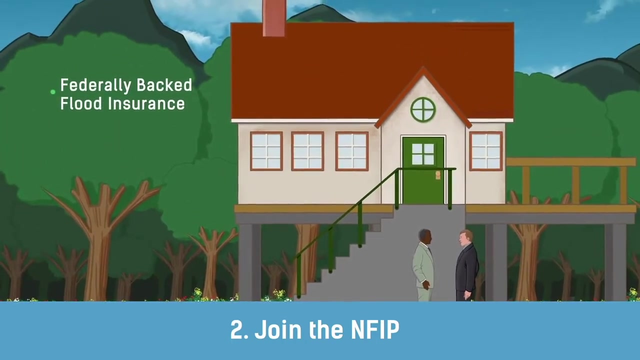 Airplanes aging infrastructure. Once you know your risks, you can begin to address them. Two: join the NFIP Not yet participating? Joining the NFIP means your residents and business owners can get federally backed flood insurance. Your community becomes eligible for.